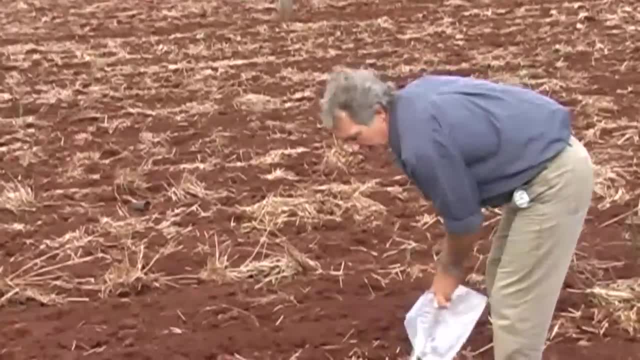 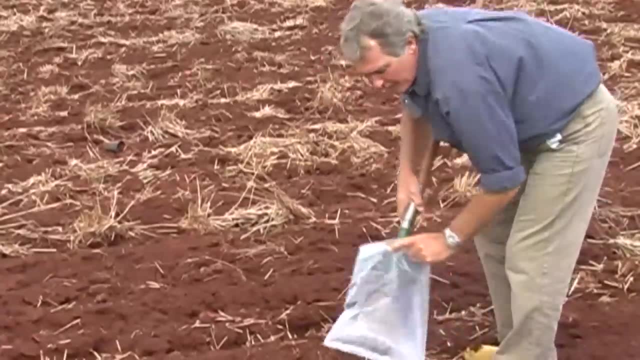 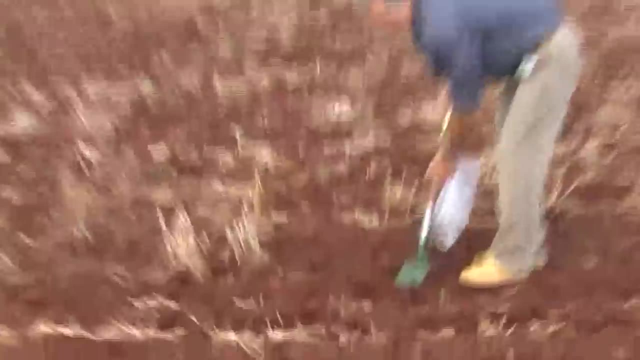 We need to get into the soil, and this is just a top soil sample here. So a little bit on the shovel down to about 15 centimetres. Then we go to another spot Not far away, Just to get a representative of the locality. 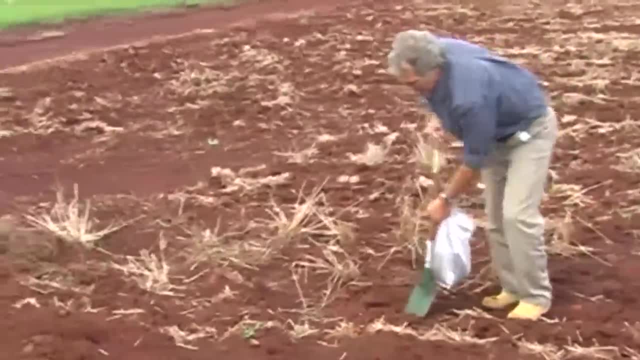 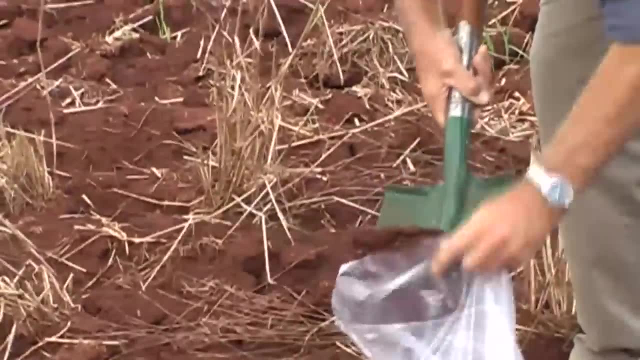 Ok, now perhaps a third spot here. This soil's a bit wet at the moment, but that'll come up really nicely. Sure SIREN, SIREN, SIREN, SIREN, SIREN, SIREN SIREN, particularly this Pratylenchus, is that it's deep in the soil. So what I've done there? 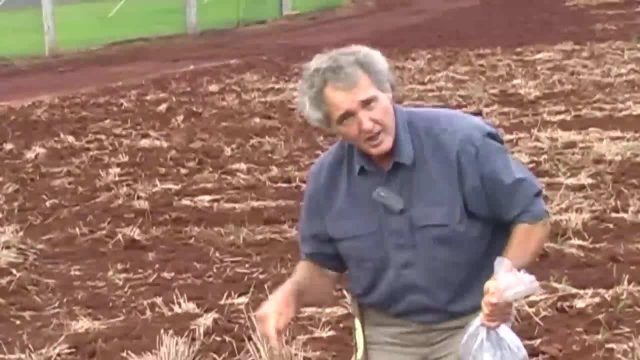 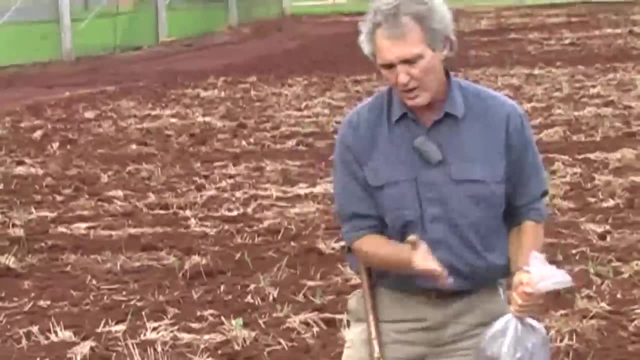 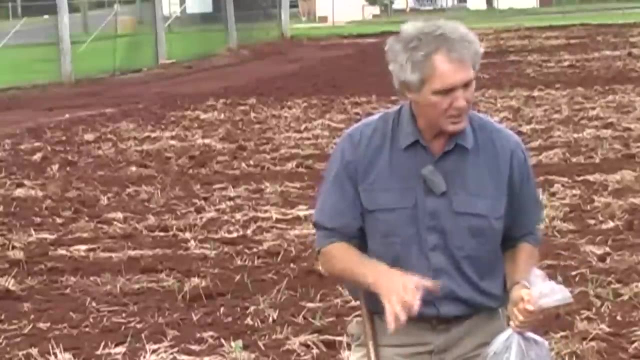 is: take a topsoil sample. the next step is to get down a bit deeper. I want to capture that subsoil sample. What can happen is when you're cultivating the soil, the nematodes are perhaps low in the topsoil and your deeper ones. deeper sample will reveal the true population. 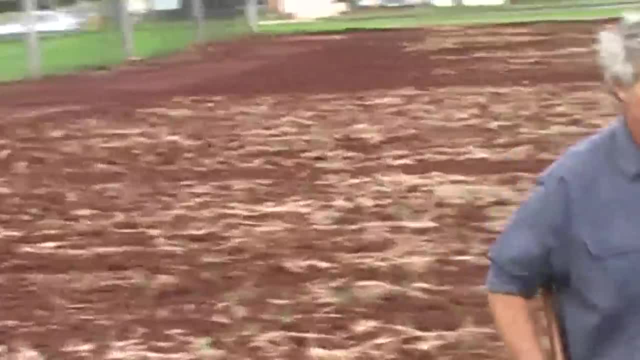 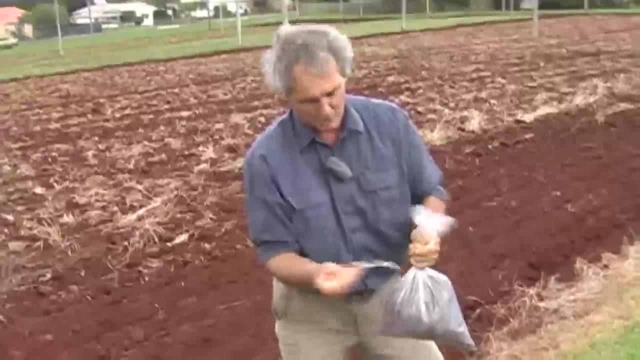 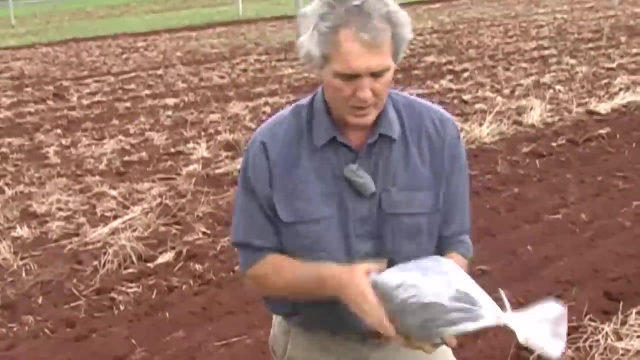 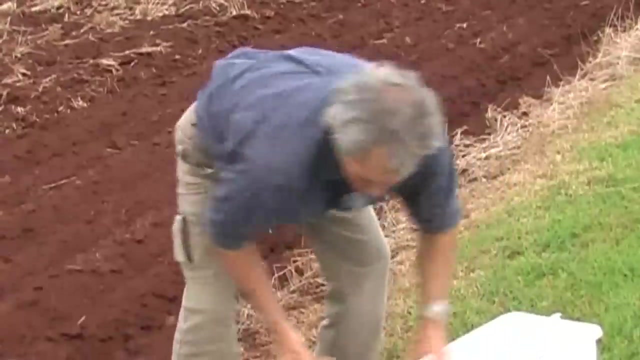 that's there. So that's your topsoil sample. We need to label that. First of all, a twist eye just to seal it. You'll note just a plastic bag- strong plastic bag that's kept the moisture in, Not a paper bag- paper bag will fall apart. A plastic bag- strong plastic bag. You'll 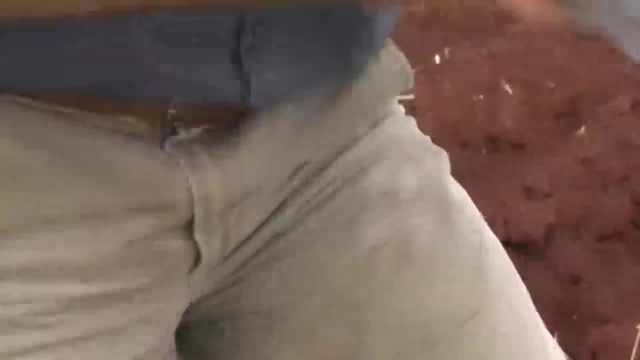 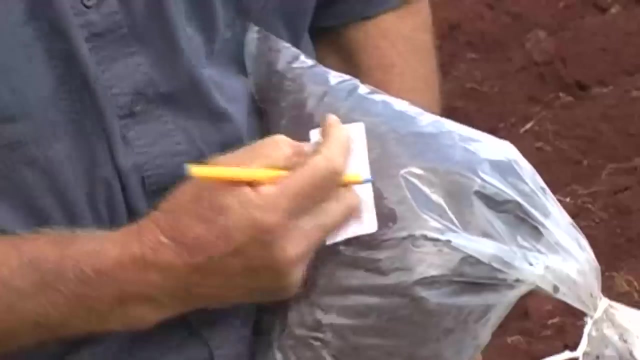 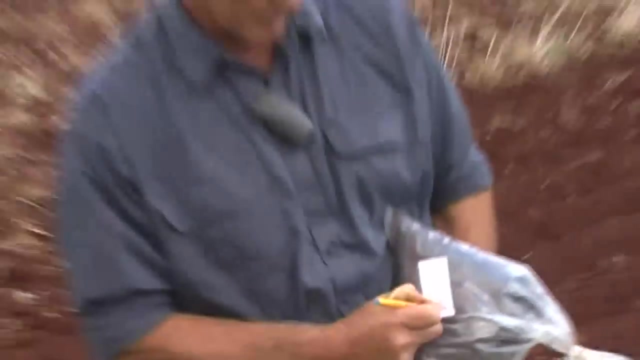 need a label on it. We like to take Speaker 1,, Speaker 2, Speaker 3, Speaker 3 samples through the paddock and we've called this one sample A. It's been three separate subsamples gone into that and that's the topsoil naught to 15 centimetres. 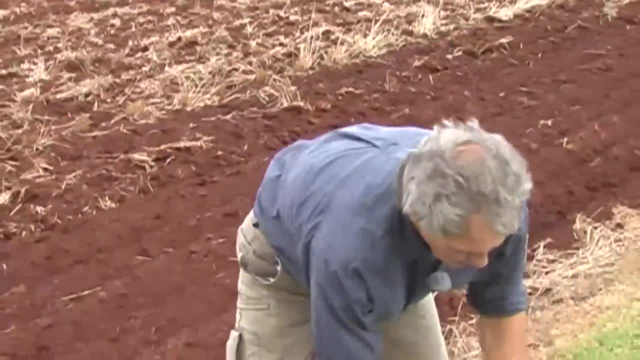 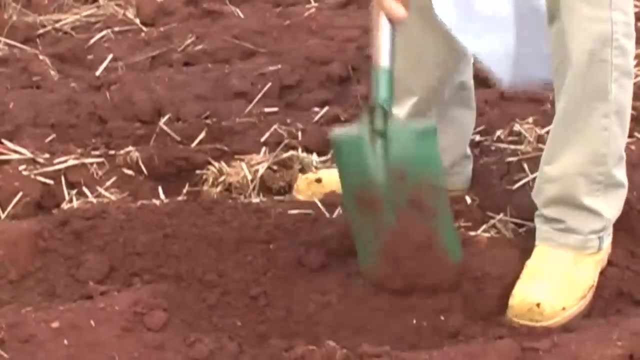 Let's go to those same spots and we'll get a little bit deeper down. This is where I started. I'll just scrape that away a little bit. I'm really getting now down into this subsoil. Speaker 1, Speaker 2, Speaker 3,. 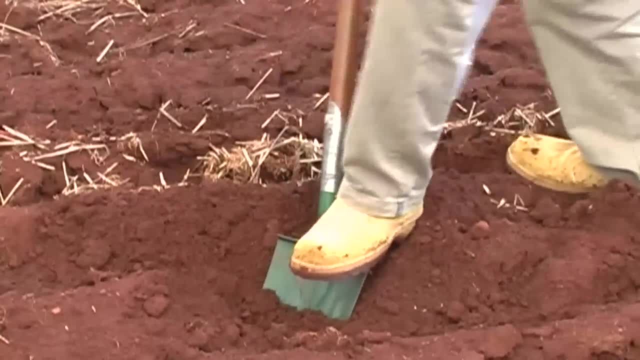 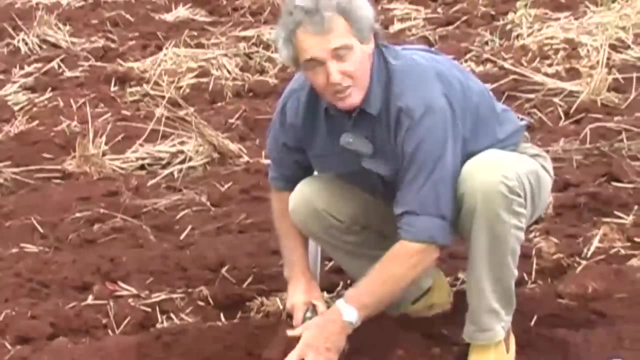 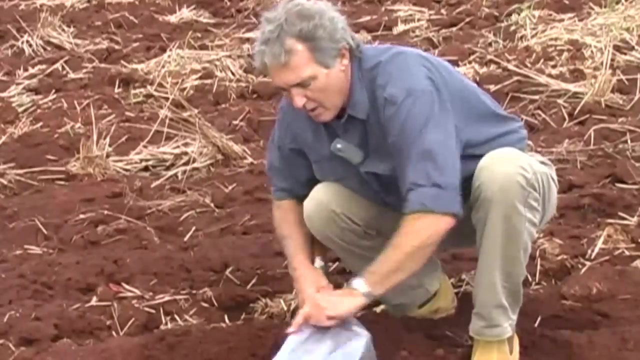 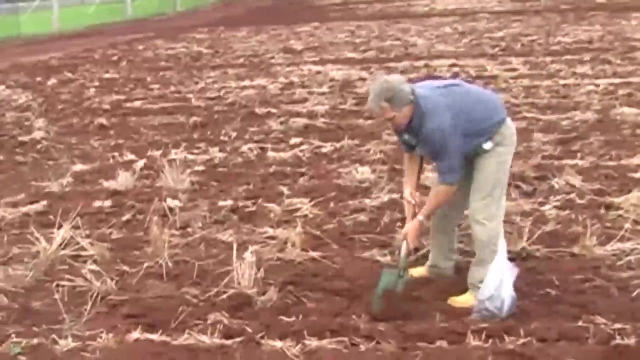 Speaker 3 sample. I mean 30 centimetres would be ideal, But right down. so you're getting a bit of this subsoil- That's the important bit- Into the plastic bag. Let's just go over here a bit further where I got the second one. I'll just scrape that soil away and then 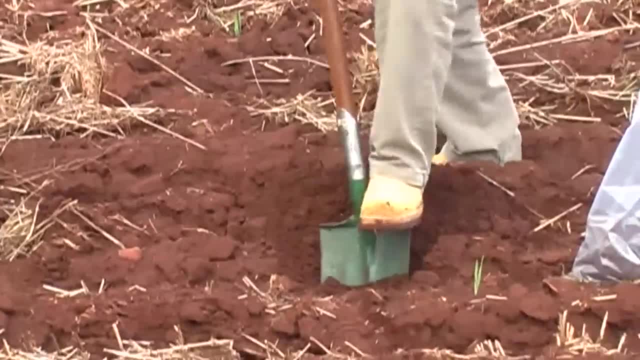 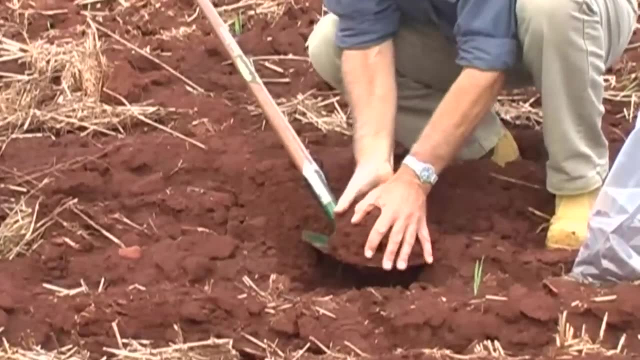 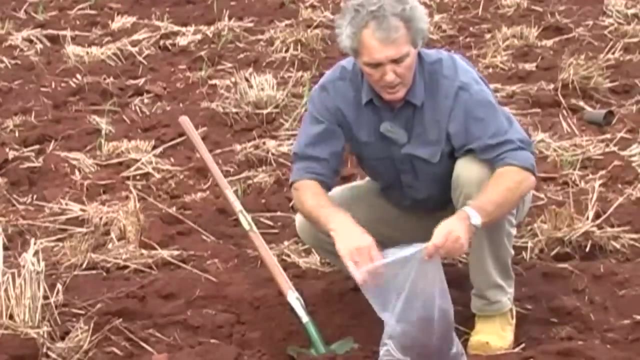 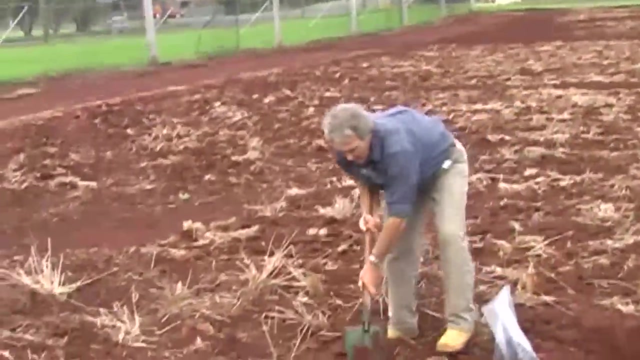 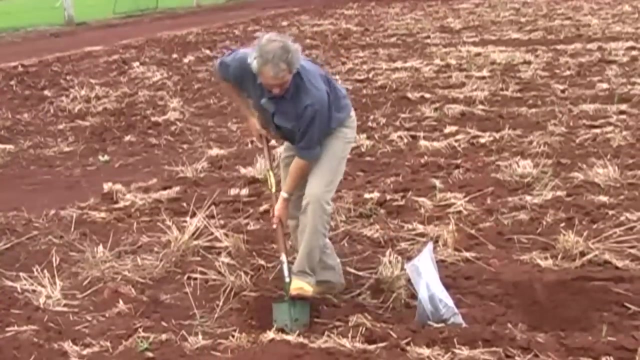 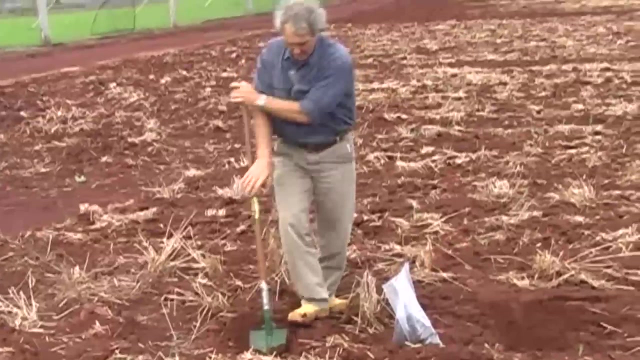 A little bit of hard work to get into the subsoil, but this is where we best look for the nematodes, down in that subsoil area, below the plough layer. And again, here's the third spot. Scrape away that topsoil where we got before and we're down into this plough layer area. 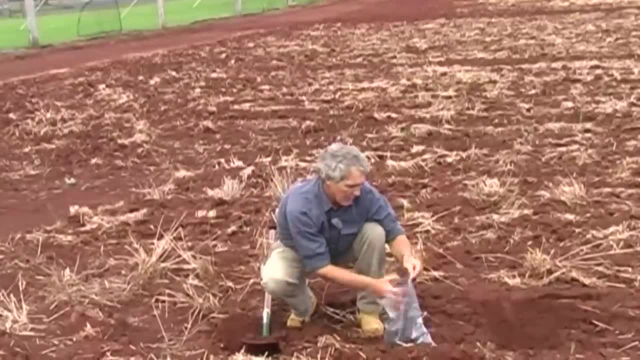 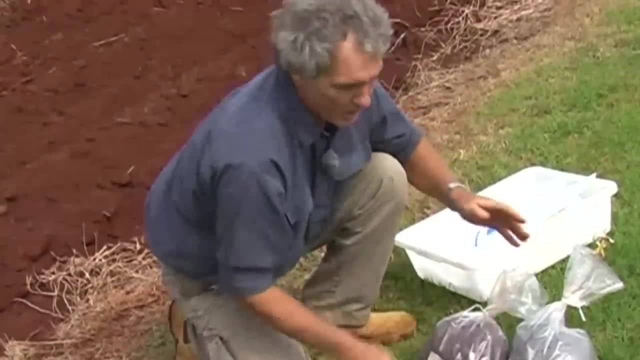 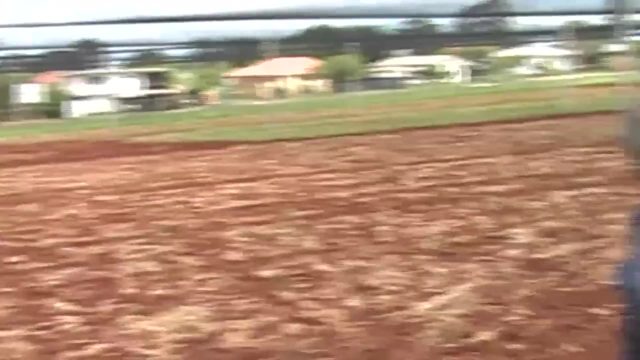 You really just need about 500 grams, I suppose. But there's probably. that's a really good sample of the paddock. That's sample A. Now, in a paddock like this we should be sampling perhaps here, but then right down the bottom and right over the far side. 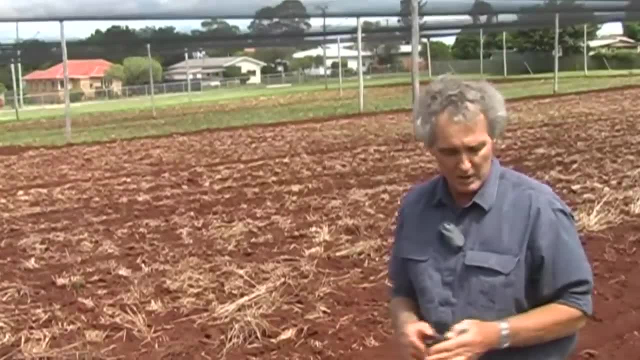 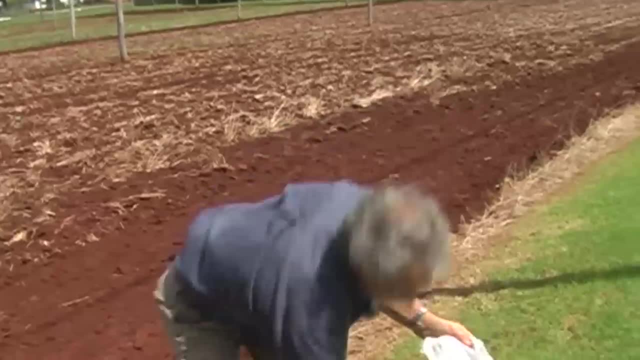 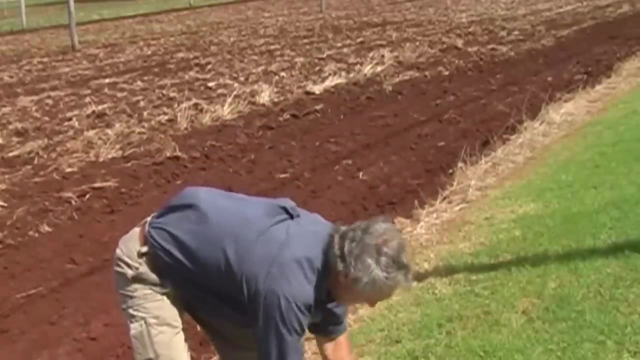 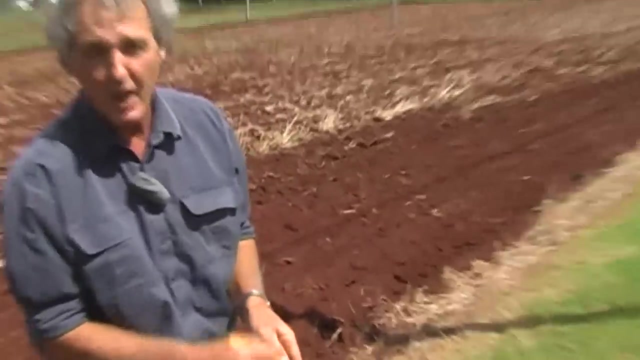 So we've ended up with samples A, B and C. We've collected our soil samples, fertilizer bag or poly bags. pretty good way to pack them in there, Just with a label around the top paddock name details your name, just to identify. 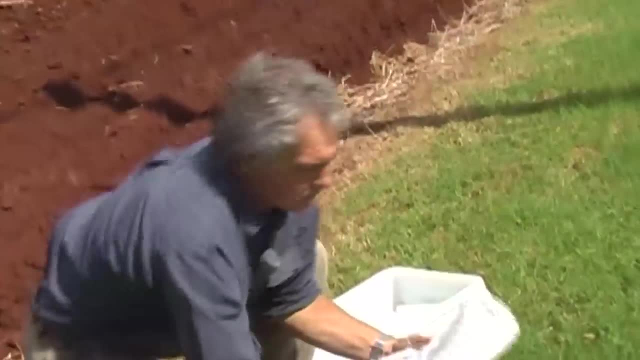 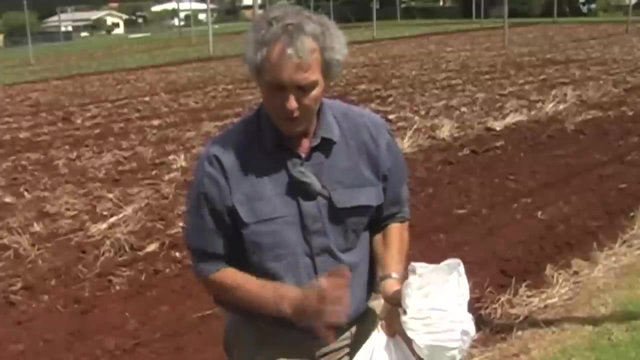 it all and just tie the bag up. Okay, that's your sample, and we need to keep this in a cool spot. Nematodes will suffer if they just throw this in the back of the ute and leave it for a couple of days. 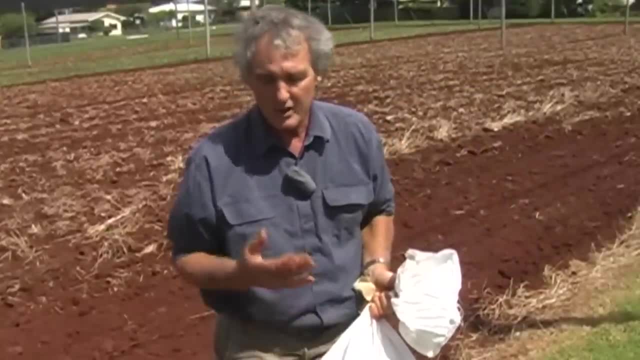 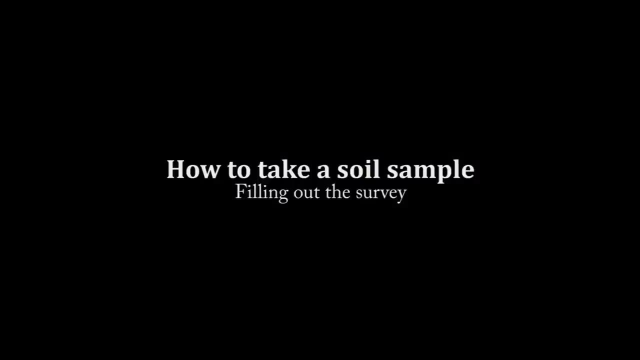 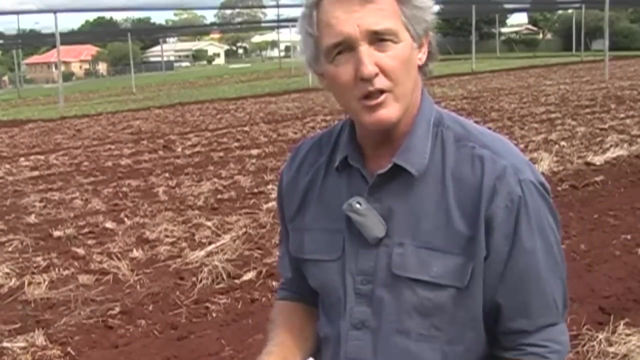 So it doesn't have to go in the fridge, It just needs to be in a cool spot and send it into the lab. We'll take it from there. A really important part of collecting these soils is to document it all. We've got a sheet here entitled test your farm for nematodes.